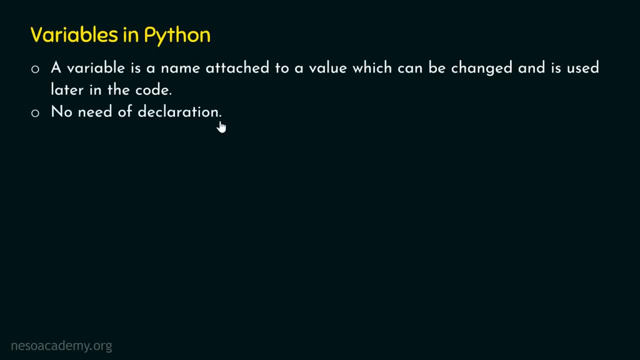 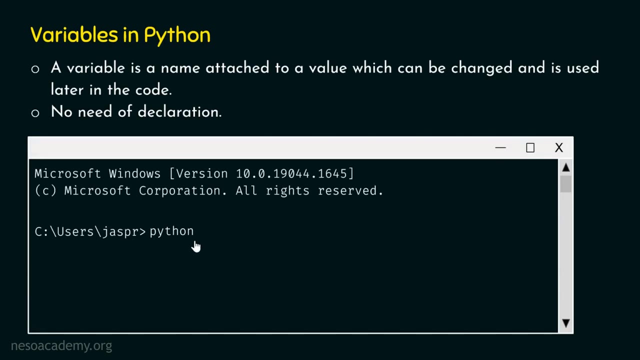 a variable before using it in Python. This is what I have written, no need of declaration. In order to understand these two points properly, we need to consider one simple example. Let's get into our command prompt and type Python, and then we need to hit enter in order to activate the Python interactive shell. 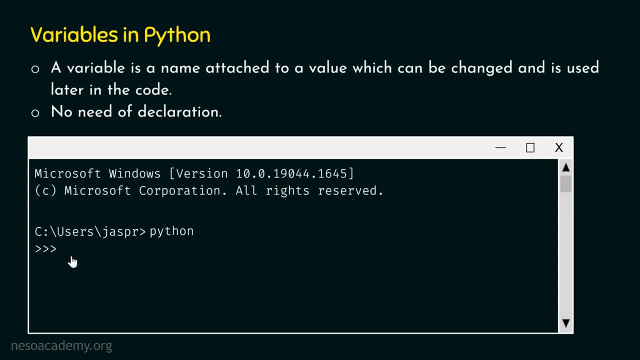 Now we are ready to type in our commands. Let's type x equal to 10.. x equal to 10 means variable x is assigned to value 10, or we can say name x is attached to value 10.. So in place of using this value directly in our code, we can use this variable x. 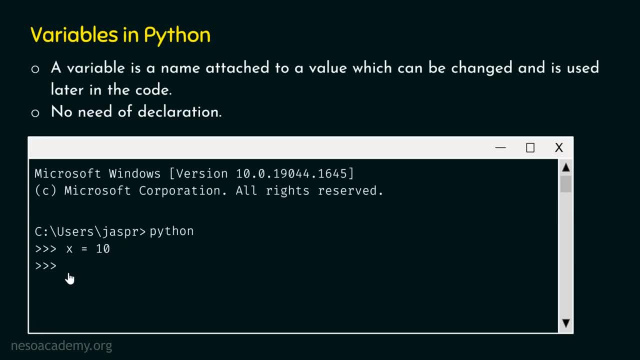 Let's hit enter and type one more command. This time I want you to type y, equal to 20.. This time we have assigned this name y to value 20.. So in place of this value 20, we can use this name y. Let's hit enter again and let's type one more command. 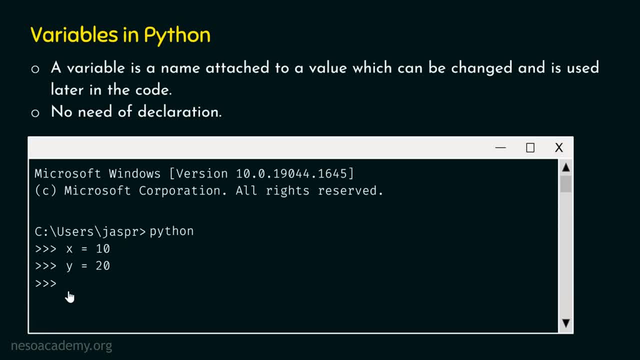 Now I want to show the power of variables. In place of these two values, we can use these names, So I want you to type x plus y: x is the name attached to value 10 and y is the name attached to value 20.. 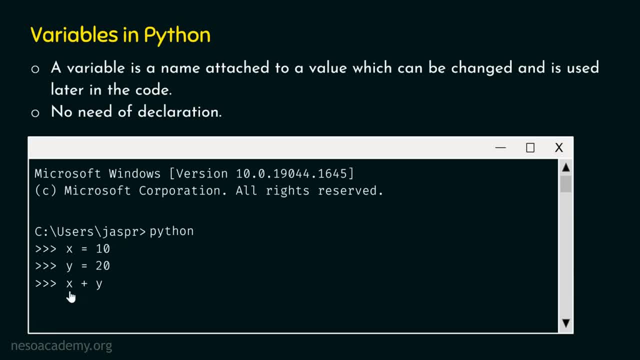 In place of these values. I have used these names, x and y, in this arithmetic operation. Here I want to add these two values, So I have not written them directly In place. I have written these variables. If we hit enter, we will get value 30 because behind the scenes, Python will replace the value. 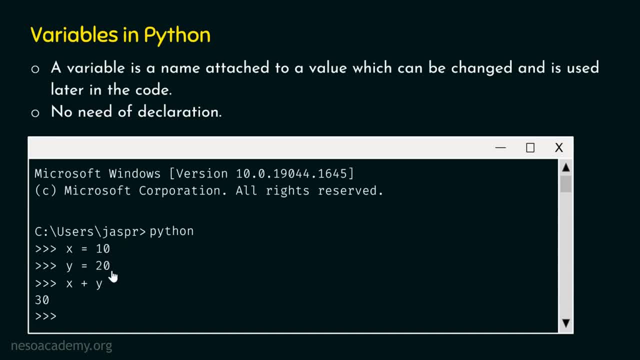 of x by 10 and value of y by 20.. This happens behind the scenes. We will not see this, how Python does it, But we know that eventually these names will get replaced by their values at runtime and we don't have to worry about it. Now, what do we mean by no need of a name? 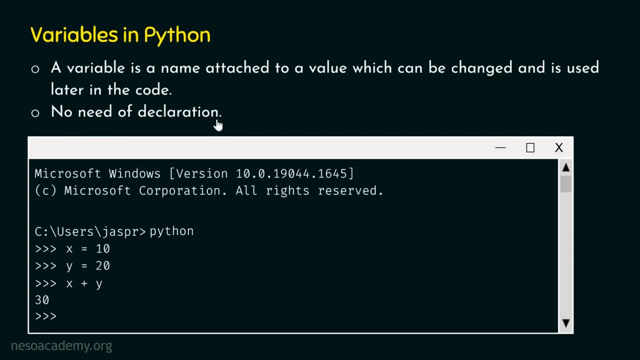 We mean no need of declaration. In order to understand this point, we need to consider how to create a variable in C programming language. In C programming language, if we want to create variable x, then we first need to declare it before using it. We cannot directly. 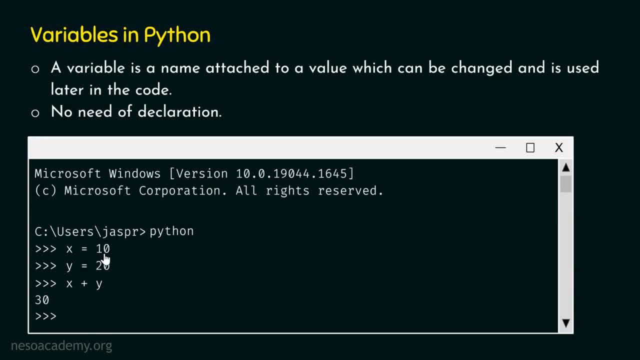 write x equal to 10.. We know that here we have assigned value 10 to x, which means that we have assigned an integer to variable x. But in C programming language we need to declare this variable before assigning it value 10.. We first need to write int x, or to be precise, we need to write int int then. 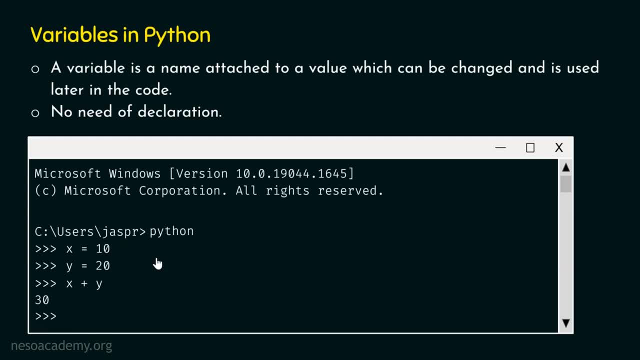 space and then x, and we need to end that statement by semicolon. In this way we can declare the variable x. Then we need to write x equal to 10.. In this way we can assign value 10 to x. You need to understand this, that in C programming language we need to declare: 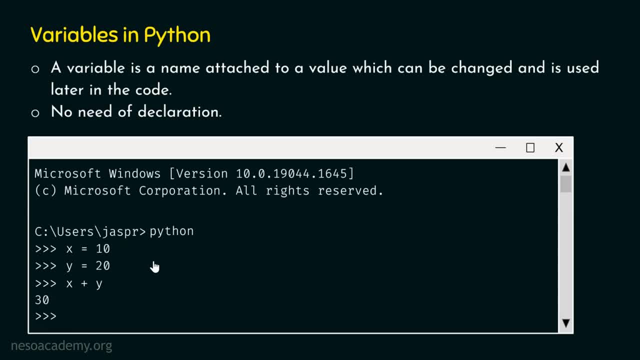 a variable. This means we need to specify the type of that variable, that is, int, integer- and then only we can assign an integer value to it. This is not the case in Python. There is no need to declare variable before using it. We can assign an integer value directly. 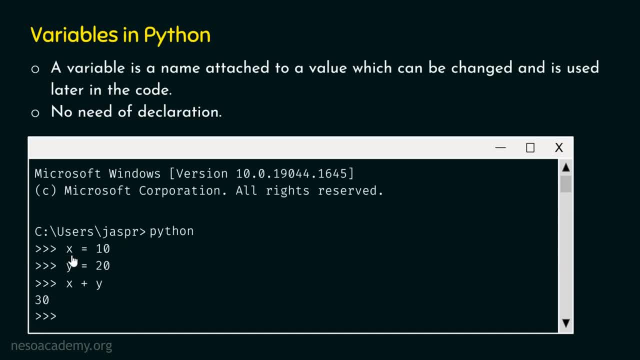 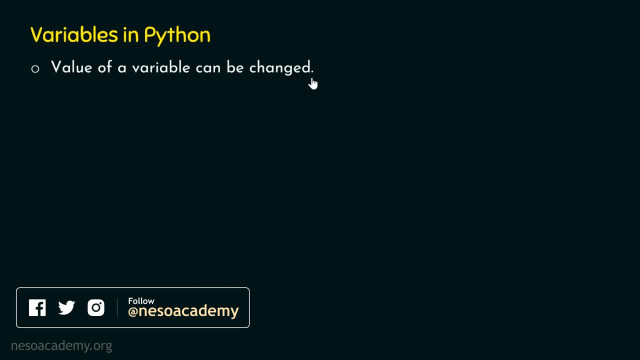 to this variable. There is no problem at all. So now you know what do I mean by no need of declaration. There is no need to declare a variable in Python. The next important point is value of a variable can be changed, Although I told this already. 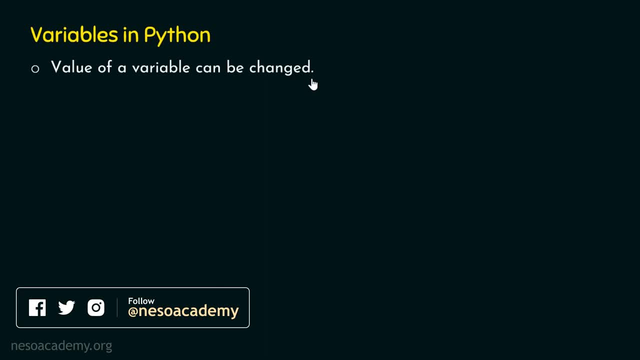 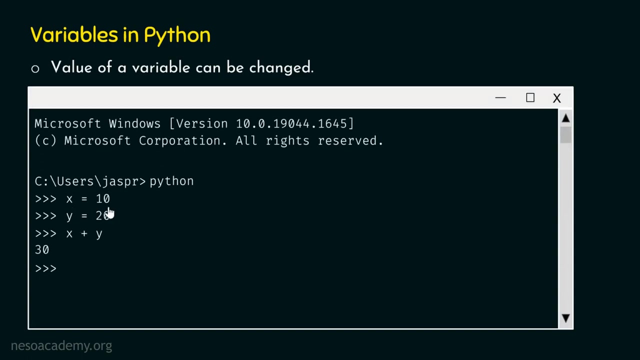 that the value of a variable can be changed later in the code, But I haven't given example for this. Now we will consider one concrete example to demonstrate what do I mean by this point. Let's consider the same example. Here we have x equal to 10 and y equal to 20.. These two variables are already created. 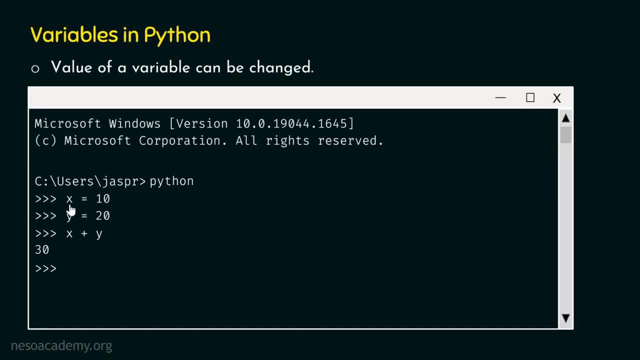 Now I want to assign a different value to this variable, x. Now, in order to see this in action, we need to type x equal to 40 in this Python interactive shell. x equal to 40 means that x is now attached to value 40 and not to 10.. This is what we need to understand. 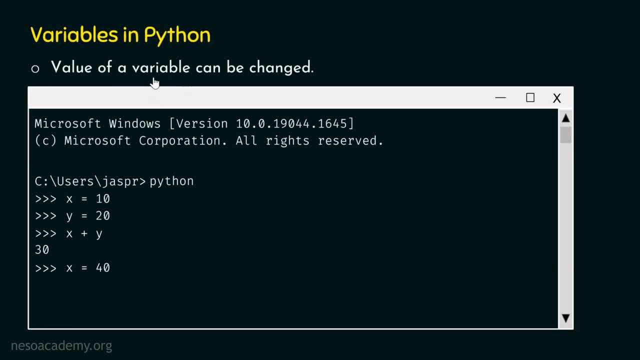 A variable has the capability to vary. That is why it is called variable- the ability to vary. So we can assign a different value to a variable without any problem. If we hit enter, we will not get any error. It is perfectly allowed to assign a different value to a variable. 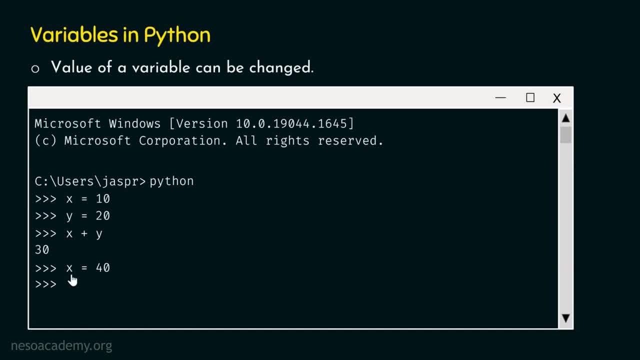 In this case, I have assigned 40 to this variable x. If we hit enter, we will again get this Python interactive shell. This means now we are ready to type in the next command. Let's type x plus y. now We know that x is now the name attached to this value 40.. So x is no longer pointing to this. 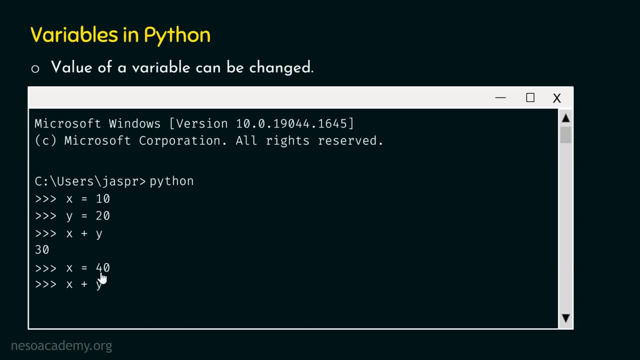 value 10.. x is now pointing to value 40. So eventually this will get replaced by 40 and this y will get replaced by 20, because y is still pointing to this value 20.. If we hit enter, get value 60 as a result, because 40 plus 20 is 60. 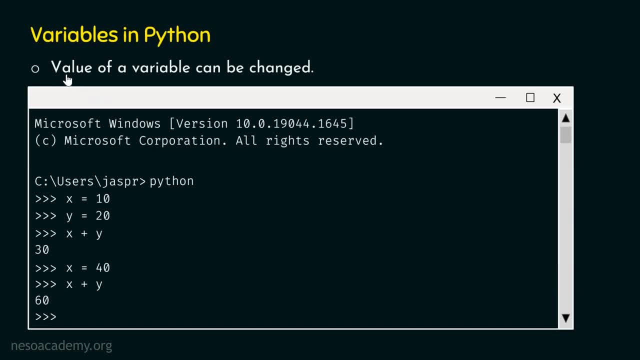 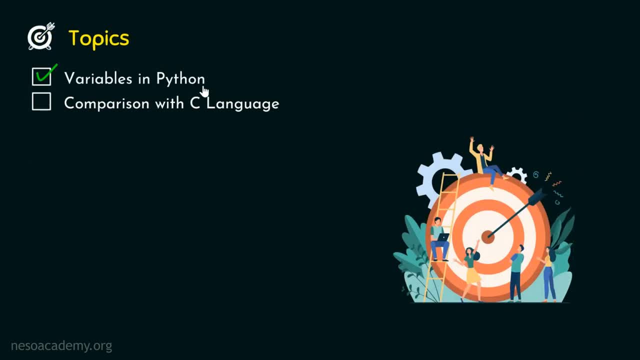 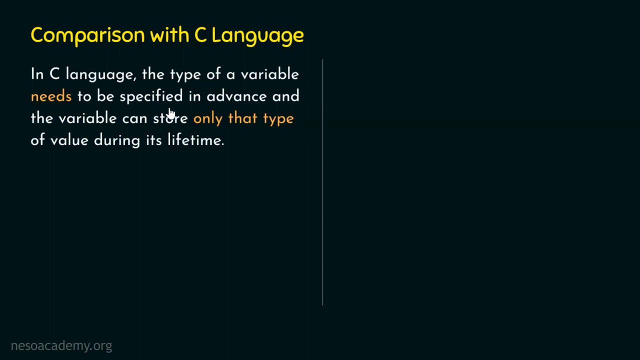 I hope this point is completely clear to you. A value of a variable can be changed. Now we are done with variables in Python. Let's move on to our next topic, that is, comparison of Python variables and C language variables. In C programming language, the type of a variable needs to be specified in advance, and the variable. 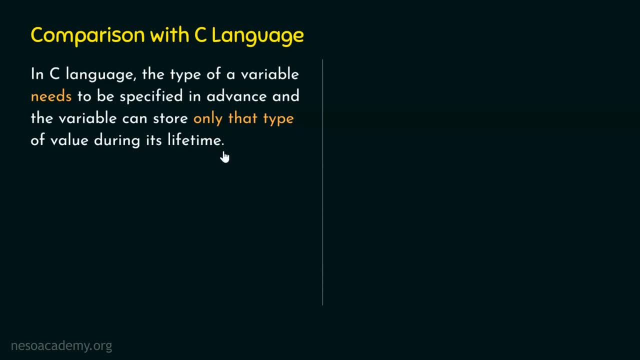 can store only that type of value during its lifetime. I told you already we need to declare a variable before using it in C programming language. This is what I have written here: The type of a variable needs to be specified in advance. Then only we would be able to use that variable in our code. 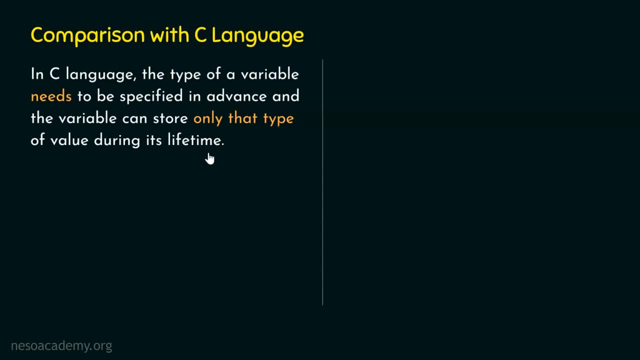 Variable can store only that type of value during its lifetime. This is very important because variables are static in nature in C programming language. Therefore, they can store only that type of value during its lifetime. Once the type of a variable is specified, that variable can store only that type of. 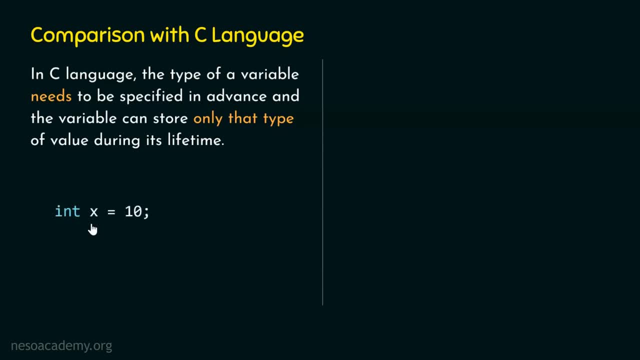 value. For example, let's say that I have declared this variable f And I have assigned value 10 to it. This variable x is of type integer. We need to specify the type of a variable in C programming language beforehand. So if we want to use this variable x, we need to specify its type. 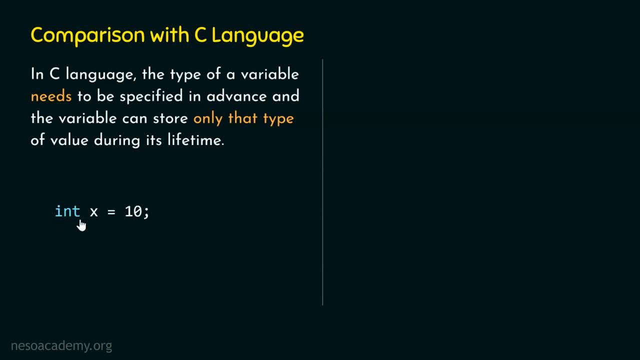 And that is why I have written int or integer in front of x, which indicates that x is a variable of type integer. Therefore, x can hold x And y can hold integer values. The type of a variable needs to be specified in advance. 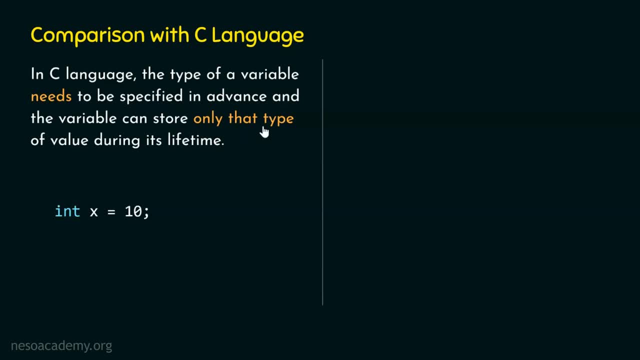 I have specified the type, And the variable can store only that type of value during its lifetime. This variable is of type integer, Hence it will remain an integer variable throughout the lifetime of the program. This means that we cannot assign a different type of value to this variable. x. 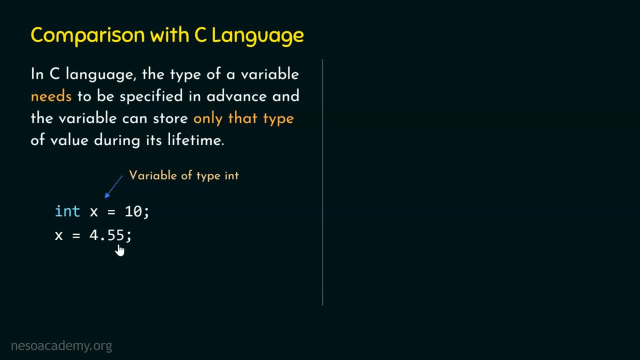 If we try to assign it, either we will get an error or we will lose precision, Like in this case. we are trying to assign a floating point value to this variable x. This is not allowed, Although we will not get an error, but eventually x will hold value 4 and not 4.55.. 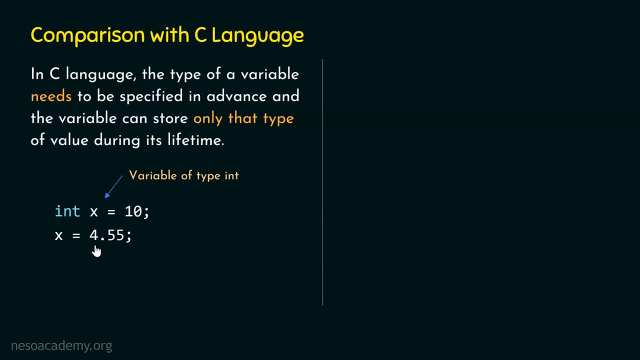 Because x is an integer variable and it can hold only integer values. Hence it is not allowed. Hence we will lose precision. in this case, We will only get value 4 and not 4.55.. We can't store a floating point value in an integer variable. 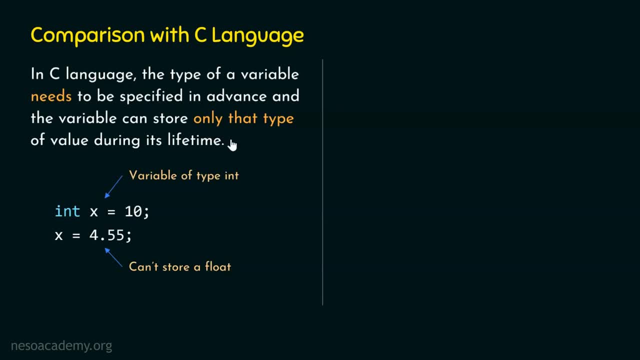 So in C programming language we can say that variables are statically typed, which means we need to specify the type of a variable beforehand and the variable can store only that type of value during its lifetime. Now let's see how Python variables are different from C variables. 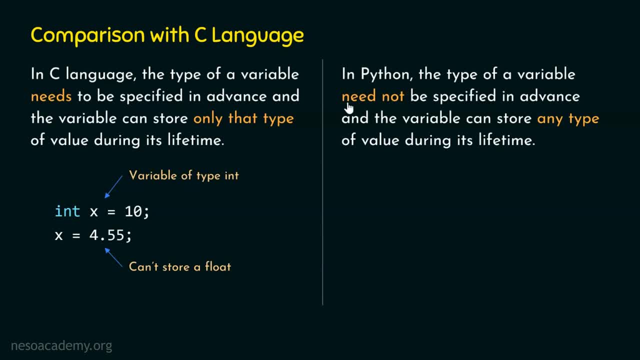 In Python programming language, the type of a variable need not be specified in advance and the variable can store any type of value during its lifetime. If you observe the statement carefully, this statement is totally different from the statement. Just an opposite to the statement. 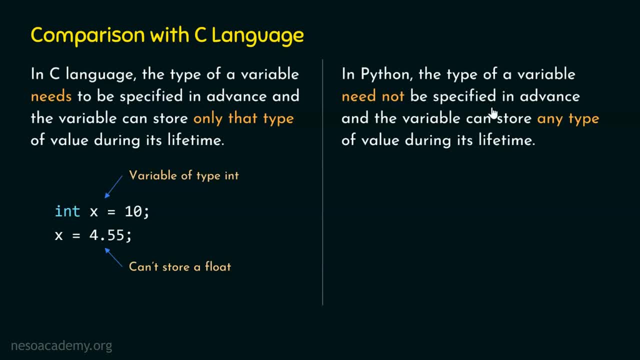 In Python, The type of a variable need not be specified in advance. The type of a variable will be known at runtime. Python will automatically get the type by seeing the value stored in that variable. This is called dynamic typing, And the variable can store any type of value during its lifetime. 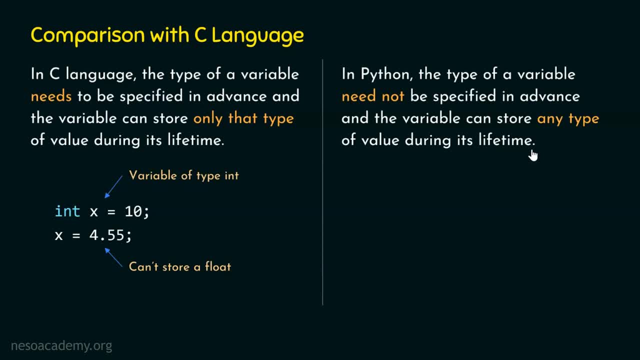 Because the type will be known when we run the code. we can assign any type of value to that variable. For example, we can write x equal to 10 without the need of specifying the type of this variable. The type of this variable will be known by Python by seeing the value which it points. 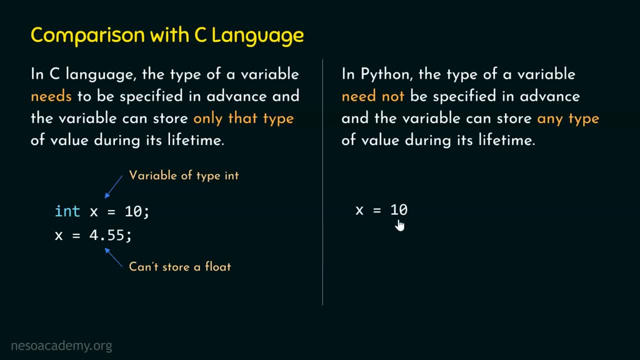 to X is pointing to this value. This value is an integer value, Hence the type of this variable is integer, But we haven't specified this type. The type is known at runtime. If we write x equal to 4.55, now x is pointing to this new value. 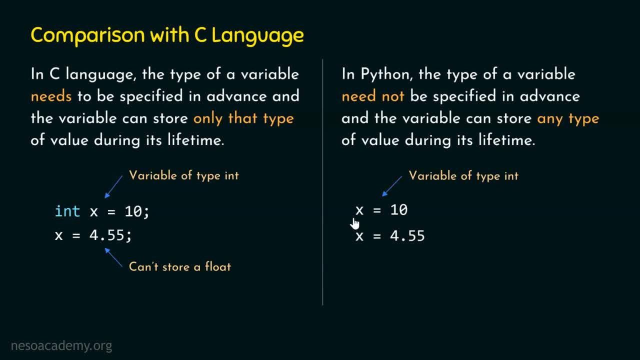 And because of dynamic typing, because the type is not static, we can assign this value to this variable x. This is perfectly allowed in Python programming language. We can assign a floating point value to an integer variable, Although now this is not an integer variable. 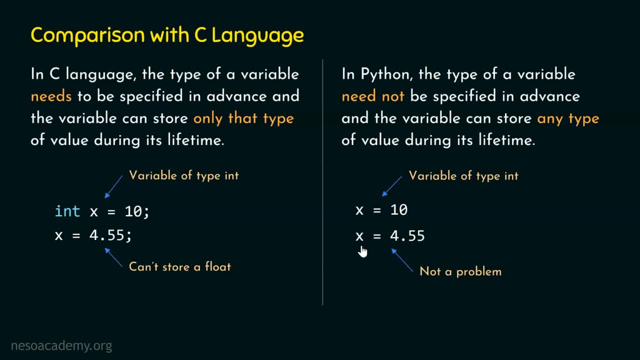 This is now a floating point variable, So types are dynamic in nature. Type of a variable can be changed throughout the lifetime of a program. Now we know the difference between C programming language variables and Python programming language variables. In C programming language variables are static. 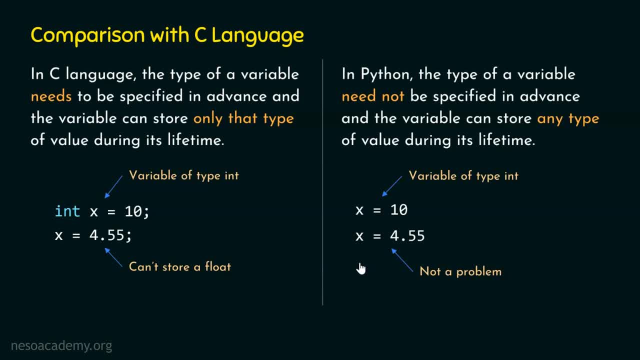 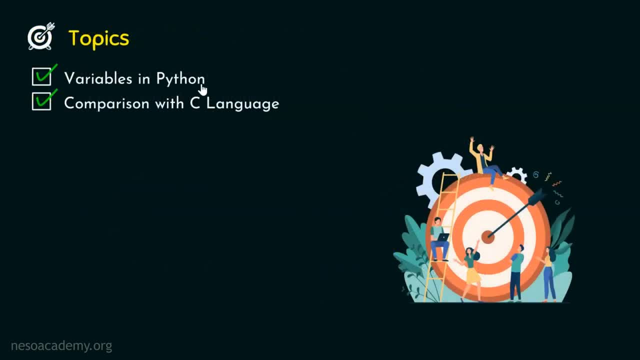 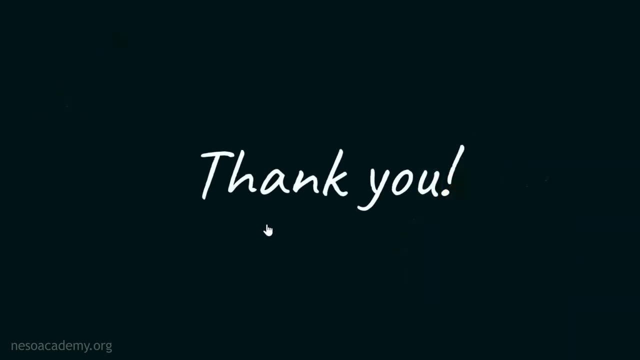 In Python programming, language variables are dynamic. I hope this point is clear to you. So we are done with these two topics. Topics: variables in Python: comparison with C language. This means we are done with this lecture. Okay, friends, this is it for now.